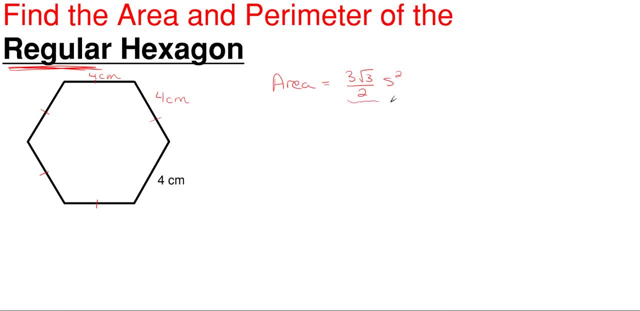 regular hexagon. Well, we're going to simplify this portion down a little bit, And then the s squared s is going to be the length of your side. Since it's a regular hexagon, it does not matter which one you use. They should all be the same. So this area is going to be equal to well. three: 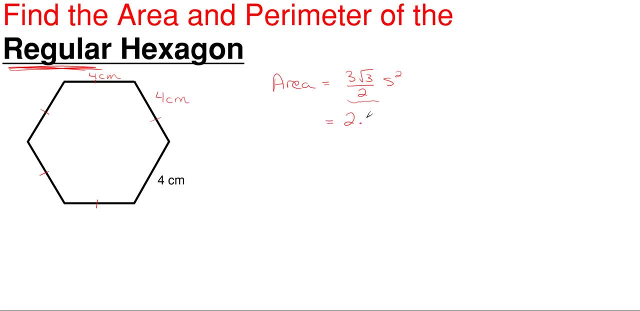 times the square root of three over two pops out to be 2.5981.. And this will be times your side. times your side again. Well, in this case, four centimeters is just the length of our side. So let's go ahead and plug. 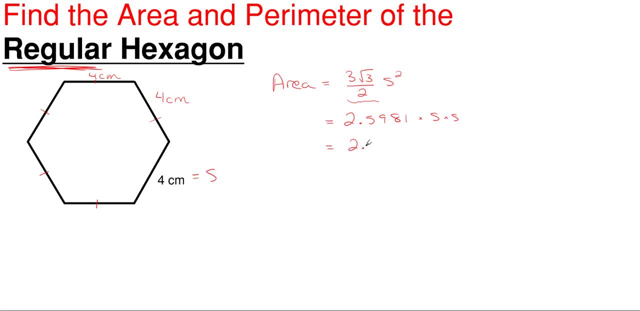 that in for s. So the area of this regular hexagon would be 2.5981, which this 2.5981 will always be that value for a regular hexagon, times four centimeters, times four centimeters, And this gives us a total area of 41.57 centimeters squared. 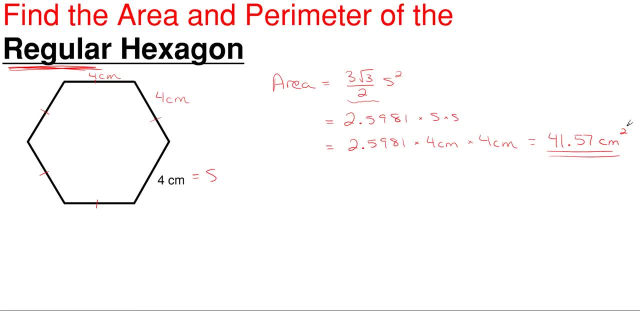 Keeping in mind that for the units you will have to have squared on whatever dimension you have. Whenever you see this little squared symbol up here, that means you're dealing with an area parameter. So our total area for a regular hexagon is 41.57 centimeters squared. Alrighty, so next we 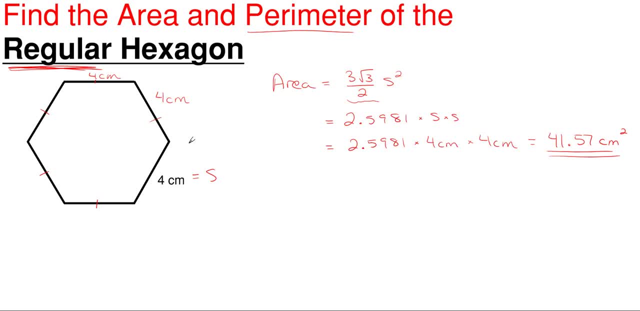 have to do the perimeter. Well, the perimeter is just a fancy way of saying how much does it take to get all the way around this shape? and back to your starting point. Since we have six sides here, we are going to be adding six numbers together. So our perimeter. 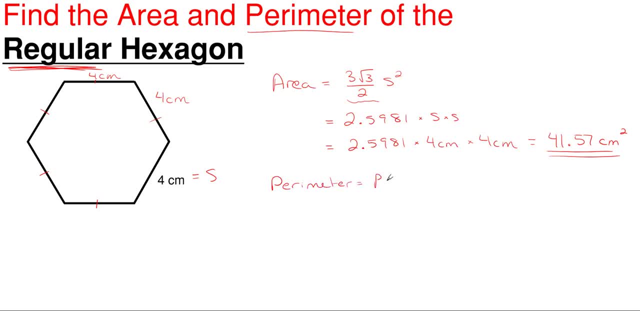 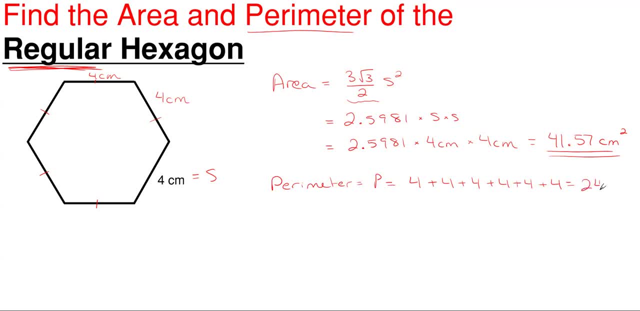 fours here, and that adds up to be 24 centimeters. Another way that you could also do this is that, since it is a regular hexagon and all the sides are exactly the same, you can just take the number of sides that you have, which is six for a hexagon.